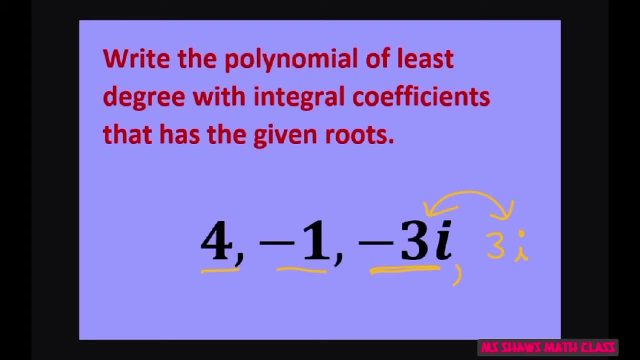 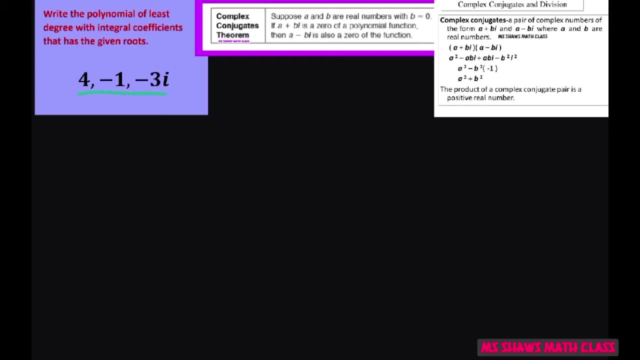 Because these go in pairs. Alright, so there's our four roots we have, So I'm going to write our factors, since these are the roots as x minus 4, times x minus a negative, 1, times x minus a negative, 3i. and again, our other one was 3i. 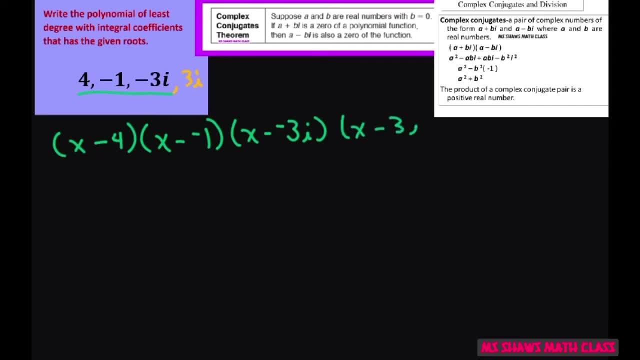 So you can write this as x minus 3i. Now the ones with the double negatives. we'll just change those to positives. So there we go Now. basically for this one. I'm going to use this formula because we have an a plus bi times a minus bi. 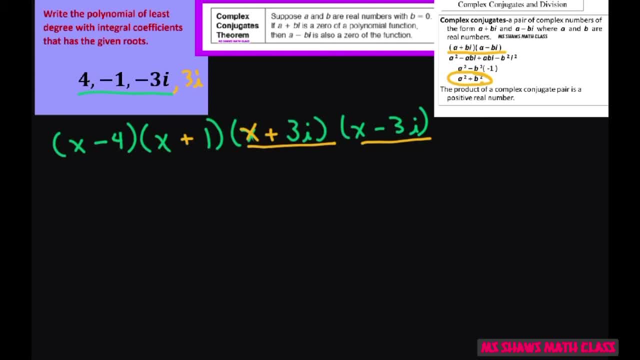 In our case, that's going to equal a squared plus b squared, where our a equals x and our b equals 3.. So this part right here is just going to be x squared plus 3 squared. Alright, so that's just going to be x squared plus 9.. 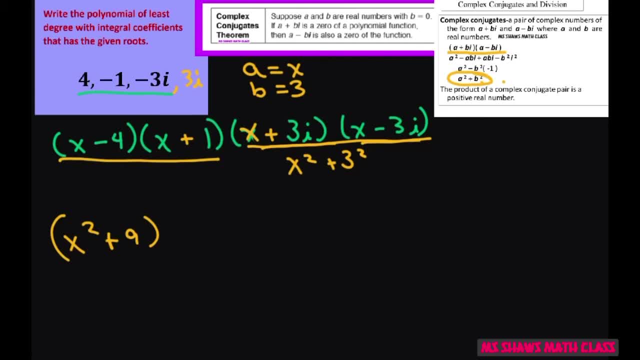 Now this piece is going to just FOIL this out or distribute it out. You're going to x squared plus x minus 4x minus 4.. You combine those so that gives you x squared minus 3x, 3x minus 4.. 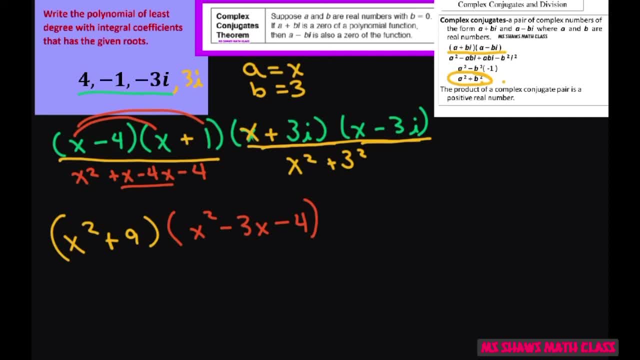 And then then we have to do the little tedious part and multiply x squared times all of that. So 1, 2, 3, that's going to give you x to the 4th minus 3x cubed, minus 4x squared. 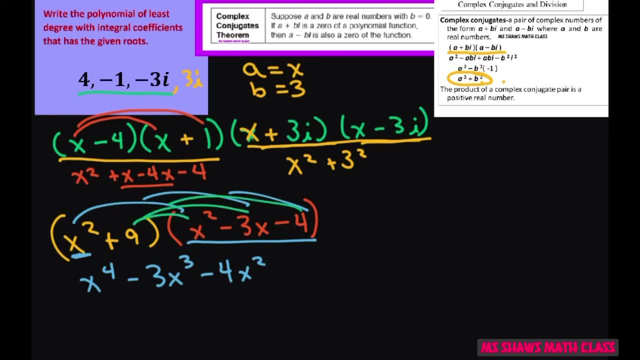 And then we're going to multiply 9 times all of that and you get plus 9x squared, Plus 6x minus 36.. Alright, and then we just have to collect like terms. So, collecting like terms, We have x to the 4th minus 3x cubed.